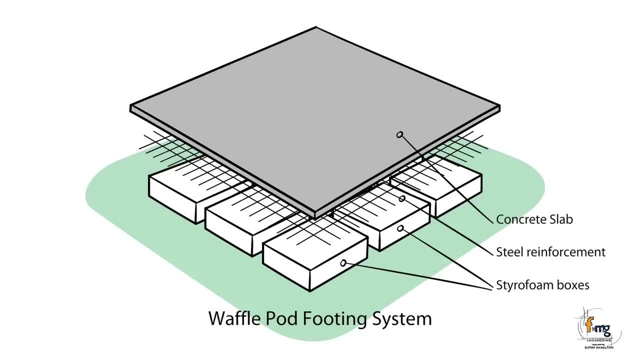 the piece can be too dim or too tight. therefore this would be a bit less efficient to build. Pros: Cheaper than conventional raft due to less concrete and steel Suitable for sites with lower reactivity. little or no excavation required. Cons: Not good for highly reactive sites. Can: 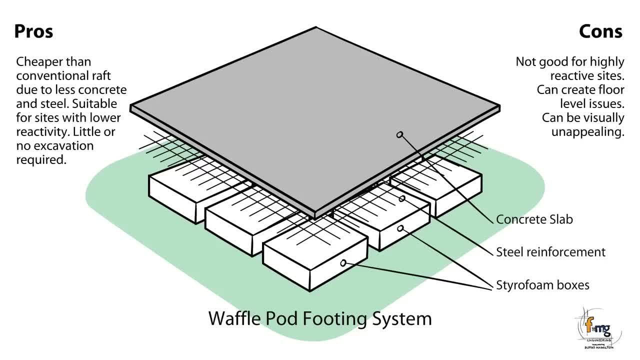 create floor-level issues Can be visually unappealing. The block footing system is a series of concrete blocks that are stacked and bear either directly on the floor or concurrently in the wall. This is the most searchable and easy way to build. This system is a pretty cheap product. You can place it in the imagination or you can buy it in an Clinic. impresivecomau A clip to check if any of these are practical. you can also purchase a sample or a sample of the product And if you have any questions about the products or a supply list, please. 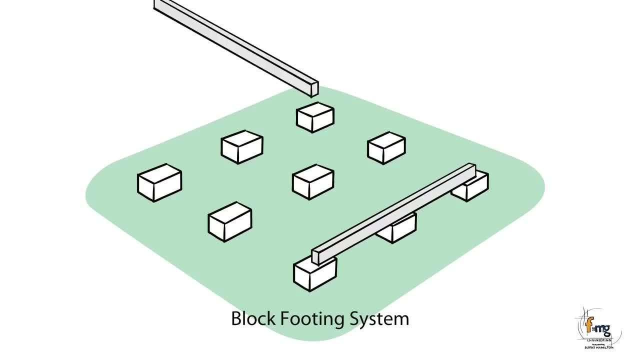 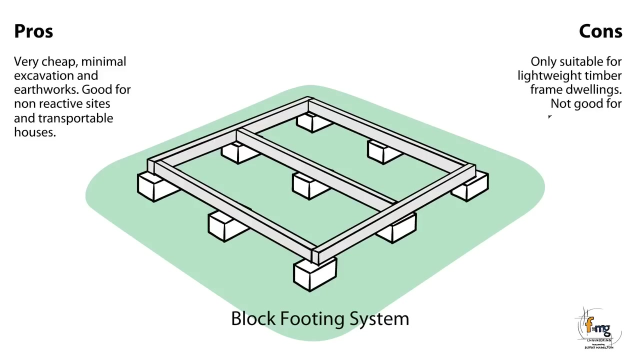 and bear either directly onto firm natural ground or on concrete pads that bear onto firm natural ground. pros: very cheap, minimal excavation and earthworks. good for non-reactive sites and transportable houses. cons: only suitable for lightweight timber frame dwellings. not good for reactive sites. floor level will be higher than outside ground level. 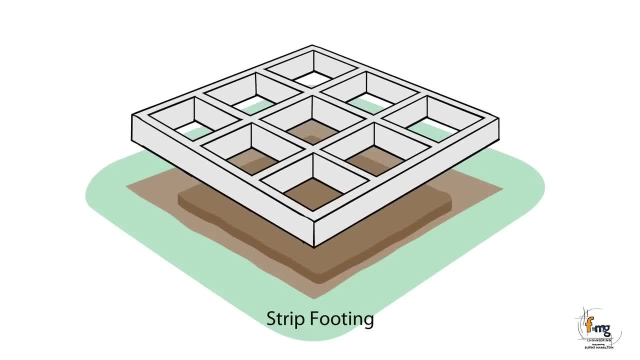 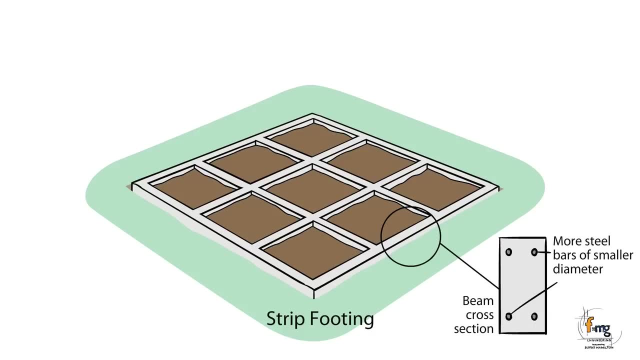 a strip footing system uses concrete beams with steel reinforcement beams can form a grid if desired to improve overall strength of the footing system. generally used to support a continuous wall or a dwelling with timber floors similar to block footings but with more strength to resist soil movement. pros cheaper than conventional raft footings. 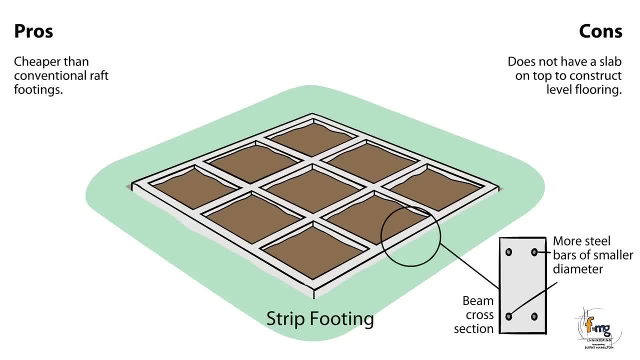 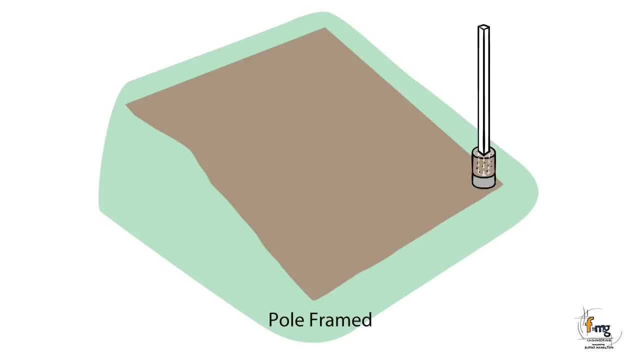 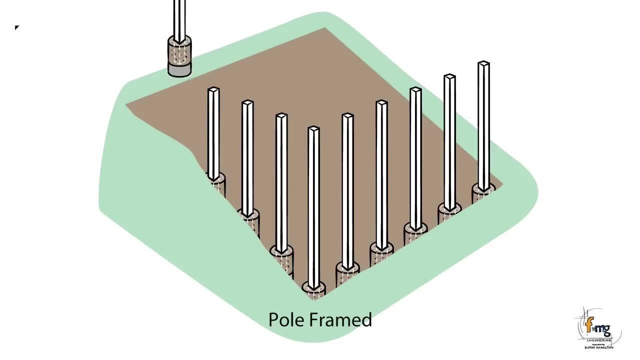 cons does not have a slab on top to construct level flooring, more prone to movement than slab footings. the pole frame is a series of poles ranging from 0.7 meters to 3 meters that support a generally lightweight structure above pros. good for steep sites. minimize earthworks on steep sites. allows for construction on. 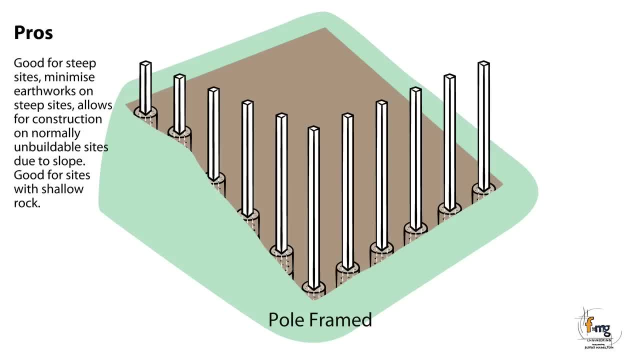 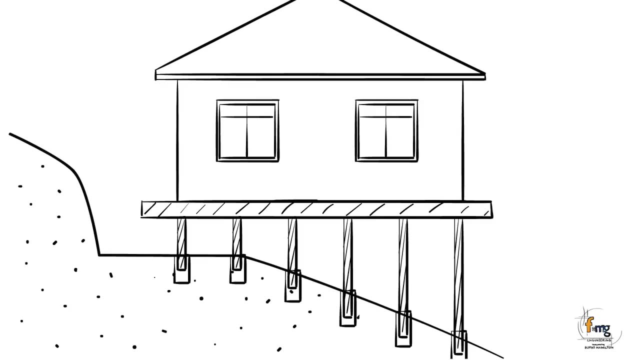 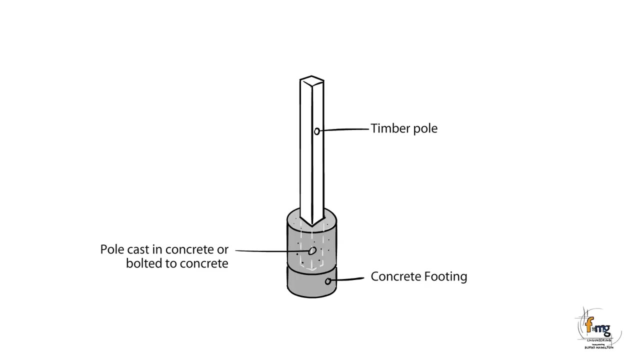 normally unbuildable sites due to slope. good for sites with shallow rock cons. generally only suitable for timber frame dwellings and therefore not energy efficient. aesthetics: not great, depending on preference. not good for reactive sites. cons: the poles bear onto a concrete footing. cons: a close-up of the pole explains how it is supported on the ground and sits on the concrete.